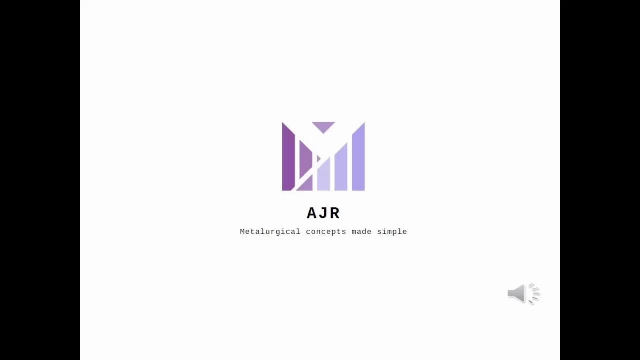 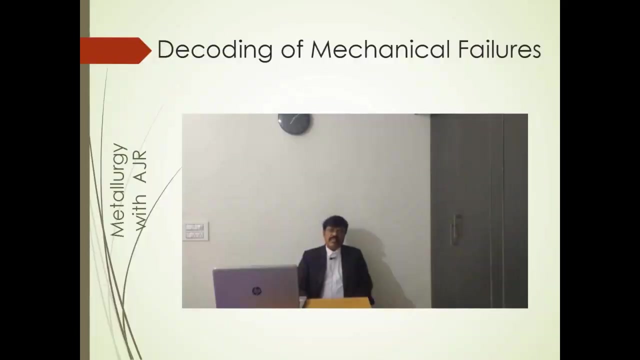 Hi viewers, welcome to metallurgy with AJR. Here I am going to meet you with a new concept, that is, decoding of mechanical failures just by visual examination of fracture surface. How is it possible When a material fails into two halves, there are two fracture surface. 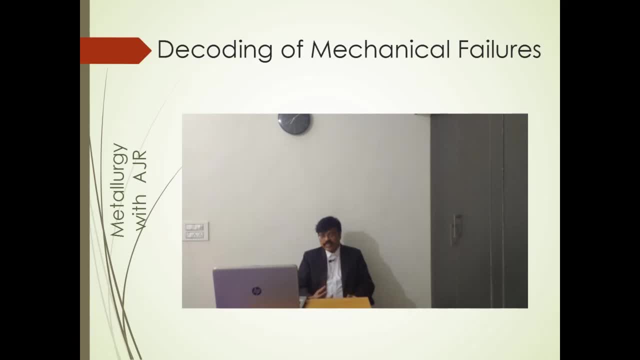 and these two fracture surface are examined visually for the various fracture features. So what are these fracture features? You are getting beach marks in the case of fatigue. You are getting chevron pattern in the case of a rapid fracture. So these type of features will give information regarding the nature of fracture. 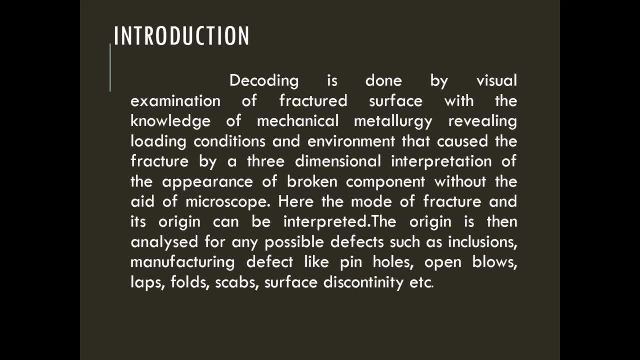 Now we can see how the decoding is being done. Decoding is done by visual examination of fractured surface with the knowledge of mechanical metallurgy, revealing loading conditions and environment that caused the fracture. by a three-dimensional interpretation, This is done by visual examination of the appearance of broken component without the 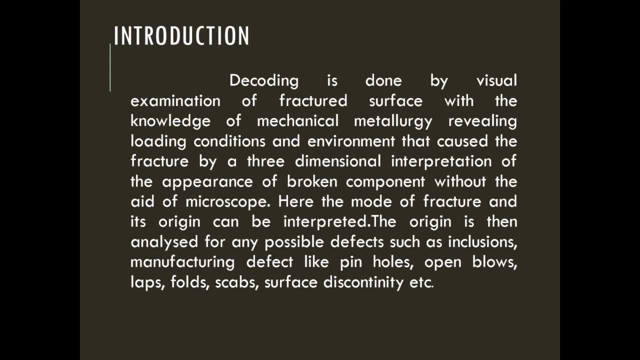 aid of the microscope. Here the mode of fracture and its origin can be interpreted. The origin is then analyzed for any possible defects, such as inclusions, manufacturing defect like pin holes, open blows, laps, folds, scabs or any surface discontinuity. 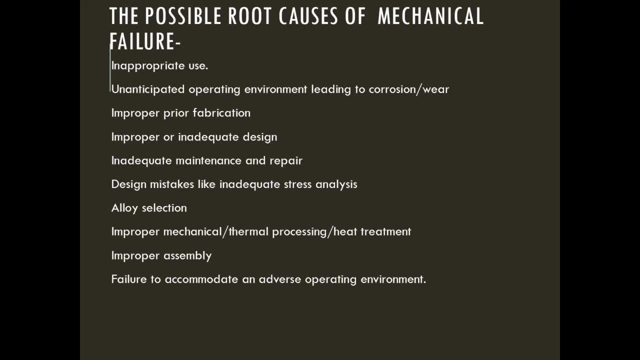 What are the possible root causes of mechanical failure? Inappropriate use, Unanticipated operating environment leading to corrosion or wear. Improper prior fabrication, Improper or inadequate design, Inadequate maintenance and repair. Design mistakes like inadequate stress analysis. Alloy selection. 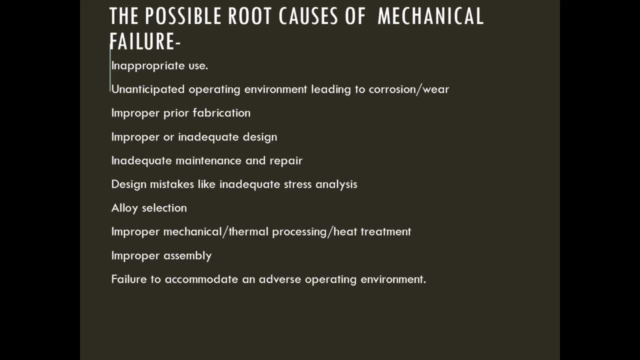 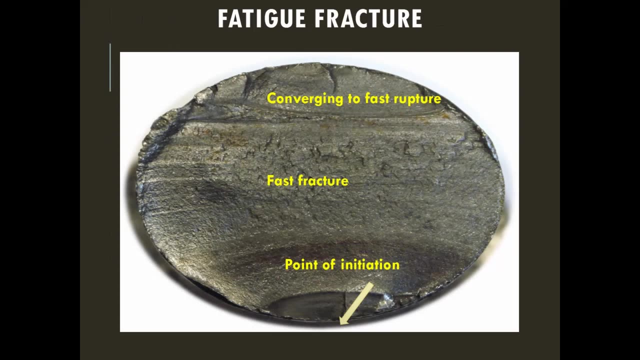 Mechanical thermal processing, heat treatment, improper assembly, failure to accommodate an adverse operating environment. This is the fracture surface of a fatigue fracture. You can see the point of initiation. The point of initiation has got a small crack of length about around 2 mm or 3 mm, and from 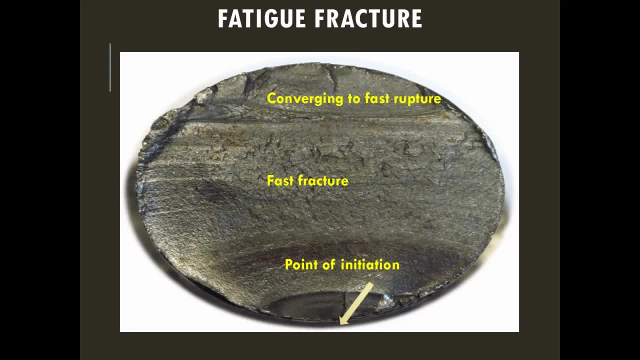 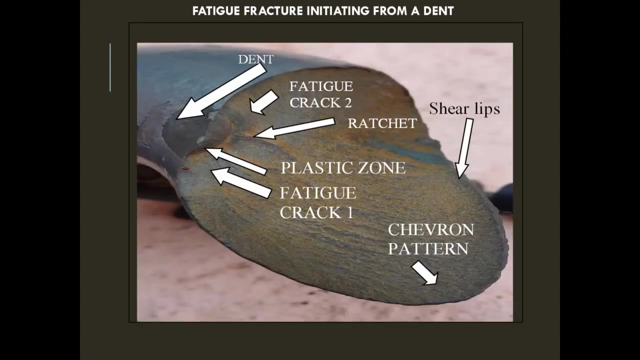 there it starts propagating. You can see the beach marks. The beach marks are the. you can see the beach marks. they are from the initiation site and then they converge again To collapse into a fast fracture, Fatigue fracture in springs. 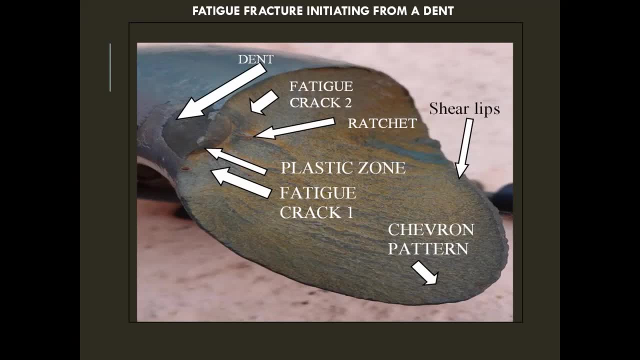 Here you can see a dent in the spring. This produces a fatigue crack. There are two fatigue cracks meeting at the ratchet. So ratchet is the midpoint of the two converging Fatigue cracks. So there are two fatigue cracks, Fatigue crack 1 and fatigue crack 2.. 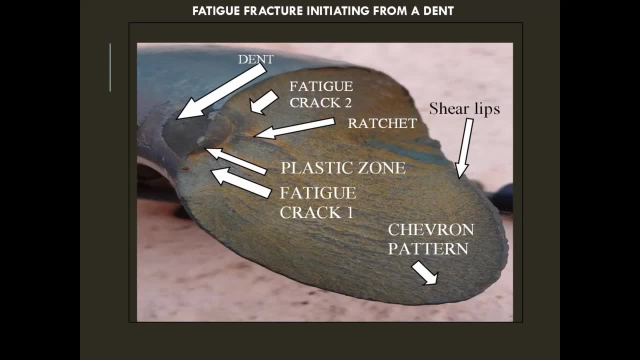 They both converge to form a ratchet. So this is the ratchet. You can see the ratchet here: The convergence of two fatigue cracks. Then afterwards the spring cannot no longer bear the load. So afterwards the spring fractures with a chevron pattern. so chevron pattern is a fast fracture. 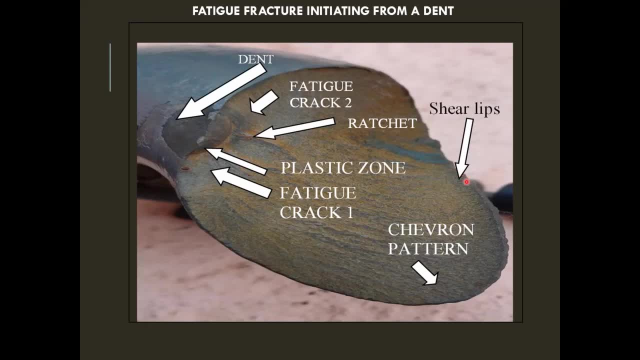 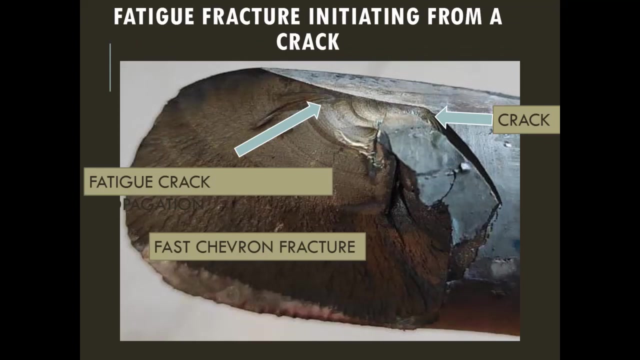 and also at the ends you can see shear lips. that means the loading conditions are very, very high. when the loading conditions are very high, then you can say that the fracture will be converted from the chevron pattern to the shear mode. so this is the case of fatigue fracture initiated from a crack on the spring. a crack got unnoticed. 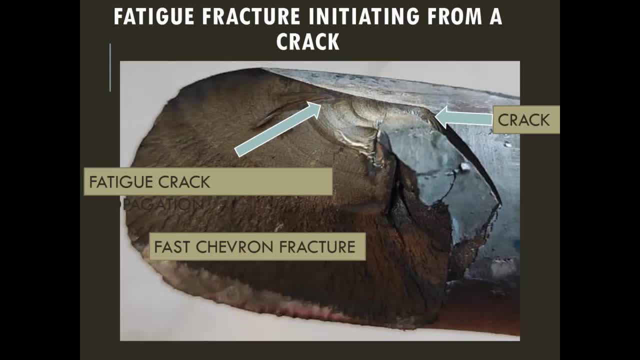 and this crack has initiated a fatigue crack. this fatigue crack is of very high magnitude and the rest of the surface is a fast chevron pattern. so normally in springs the surface property is very, very important. the surface must be without any cracks or surface blemishes or any manufacturing defects like laps, seams etc. 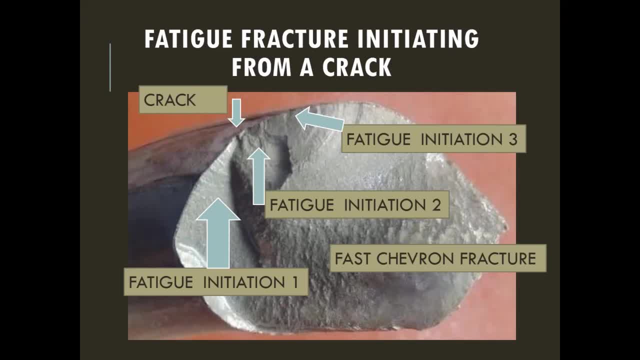 this is also another case of a fatigue crack propagating in a spring from a small crack. see here you can see a very small crack. this is the small crack. is there? this got unnoticed. so now there are three fatigue crack initiation from that particular crack point. fatigue initiation one, fatigue initiation two and 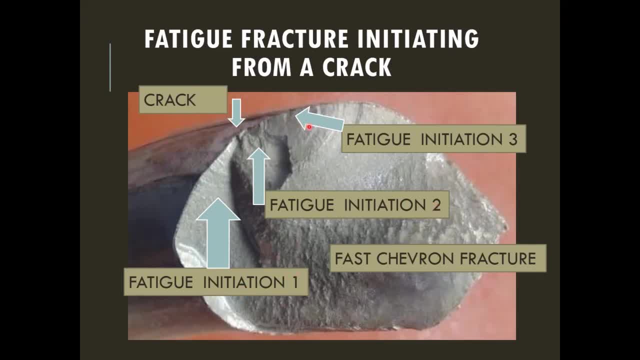 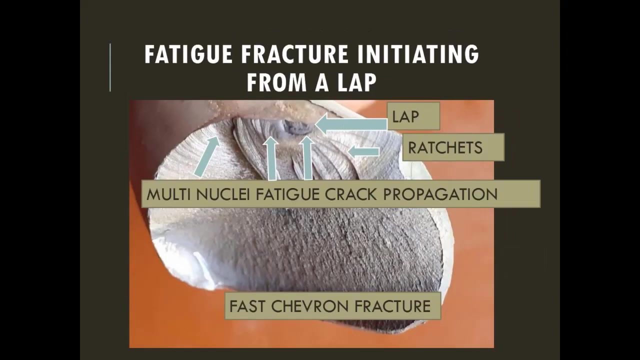 then the third one. so these two and three meets in the form of a ridge here. one and two form a ratchet here. so here you can see the ratchet. the rest of the fracture is a chevron fracture and the rest of the fracture is a chevron fracture and the rest of the fracture is a chevron fracture. 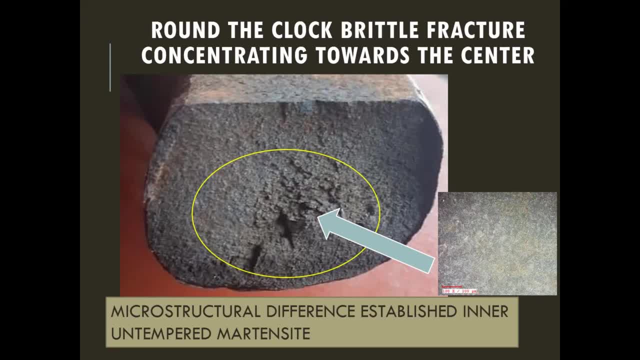 see here you can see round-the-clock brittle fracture concentrating towards the center. so this is a hundred percent brittle fracture because the material is highly brittle. see, normally the tempered martensite is will be having more amount of toughness here. untempered martensite you can see. untempered martensite means white martensite. 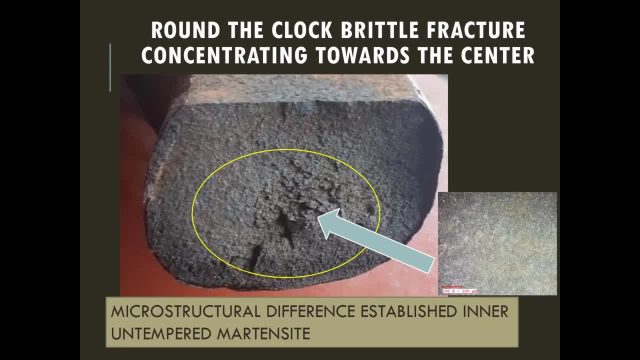 has quenched martensite. when martensite is quenched from the austenitic region rapidly you will be getting untempered white martensite. so this untempered martensite is highly brittle. its hardness also is very high. it will be around 65 rc. hence you can see this type of a brittle. 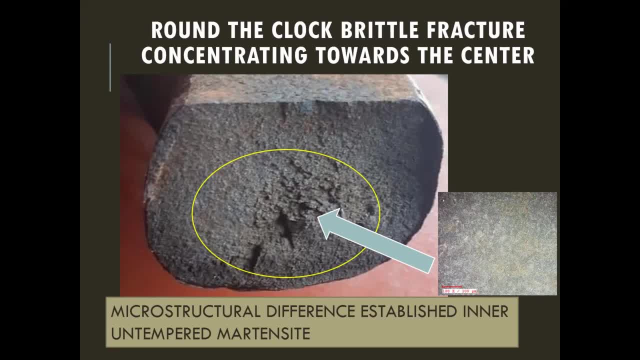 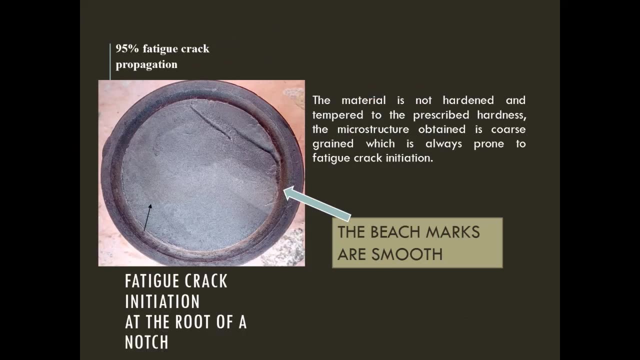 fracture around the clock- brittle fracture, that is the fracture propagating throughout the circumference from zero to zero. so this fracture is propagating throughout the circumference from zero to twelve o'clock like this. so this is a case of fatigue crack propagation in a shaft. see here the beach marks are very, very smooth. 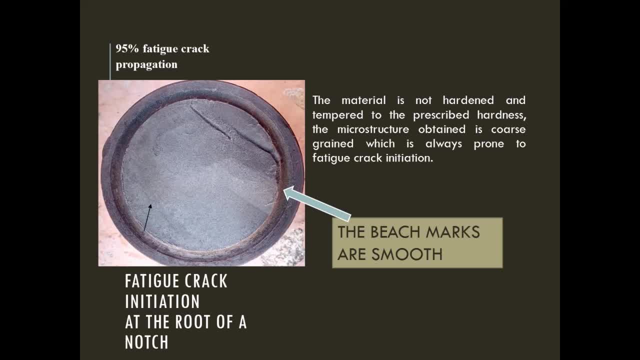 when the beach marks are very, very smooth, then you can immediately say that there is some problem in the microstructure. say the microstructure may be coarse grained, because if it is very coarse grain means normally the beach marks will be very, very smooth. it will be coming like this only. and also, one more thing is here in this: 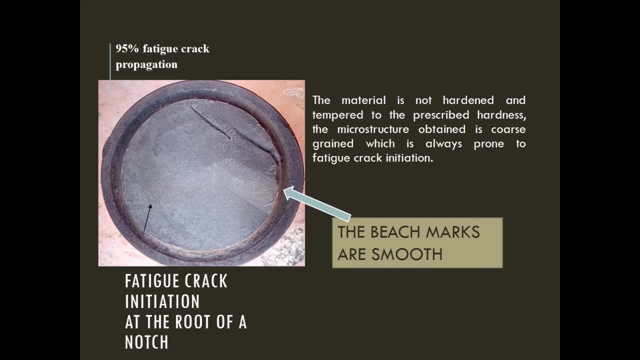 photograph you can see that the fatigue crack has propagated due to a notch problem. a shaft having a very notch, very curved notch is there, so this notch will give the notch effect on the material, so the stress intensity factor along the notch will be very, very high. so normally a fatigue crack is easy to propagate along the notch area. 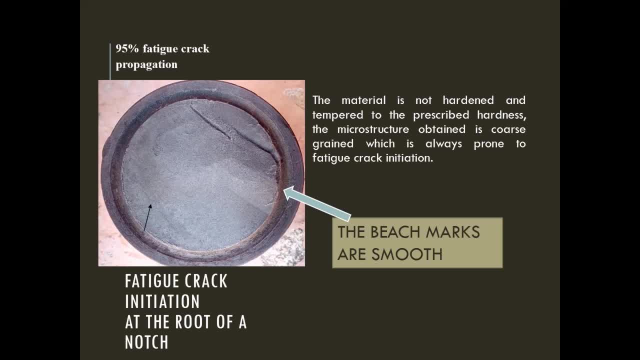 so normally what they do is in industry. they used to properly maintain the notch areas, they used to clean the notch areas. they have to see visually periodically. they have to see whether is there any fretting, because fretting is a corrosion. fretting, corrosion is very, very common in shafts. 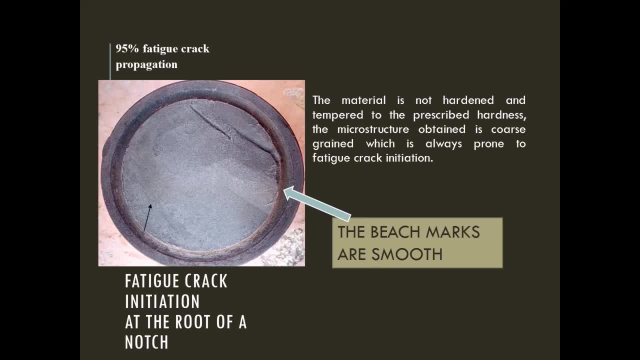 where there are journals are fitted along the notches, so there fretting corrosions are very, very common. so whenever there is a fretting corrosion, automatically what will happen. the next stage is fatigue. only the fatigue will be very, very fast. so in this case you can see that 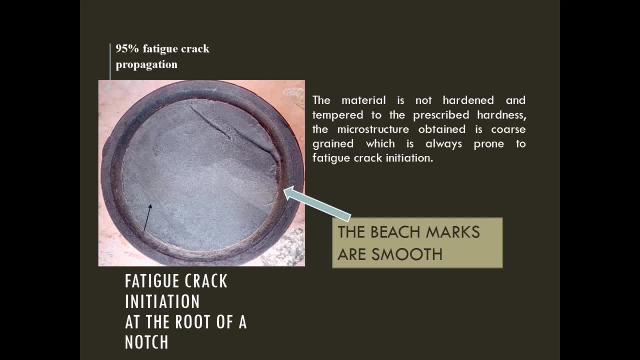 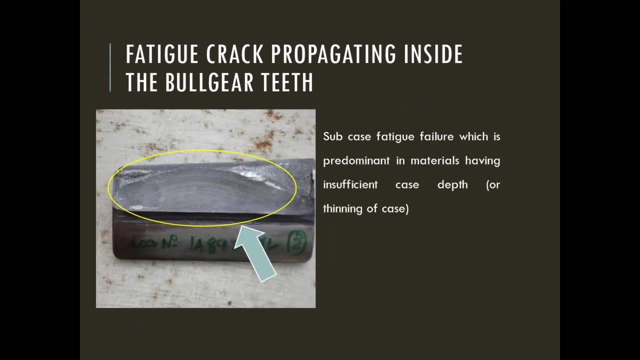 fatigue crack is very, very fast, so it is coming from one particular area to the last and in a very smooth manner that you can see the beach marks. this one is something different. it is a sub case fatigue fracture. this is a bulgir teeth. the surface is hardened to around 55 rc. 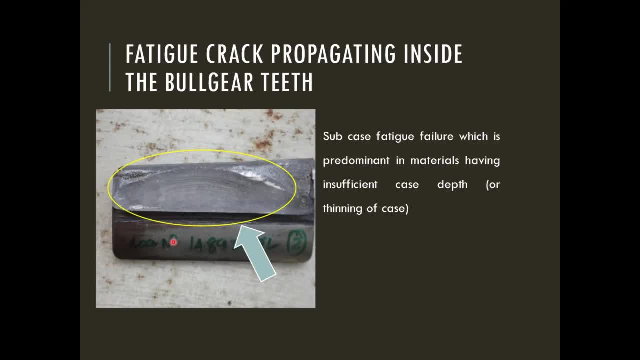 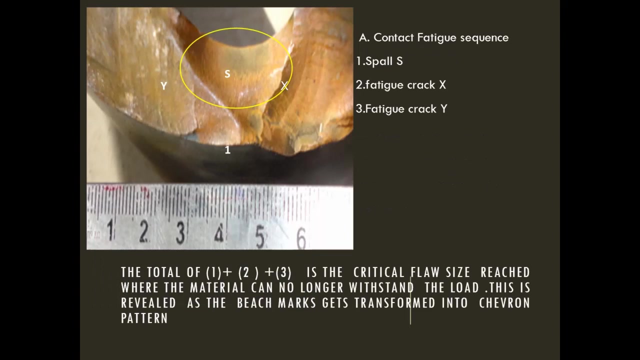 and the surface is very hard. so the fatigue rack starts propagating inside the component, inside the common. this is called sub case fatigue. this goes unnoticed in several cases. this goes unnoticed without the knowledge of the mechanical people. this is spalling in the case of some bearings. see here you can see the spalled area. 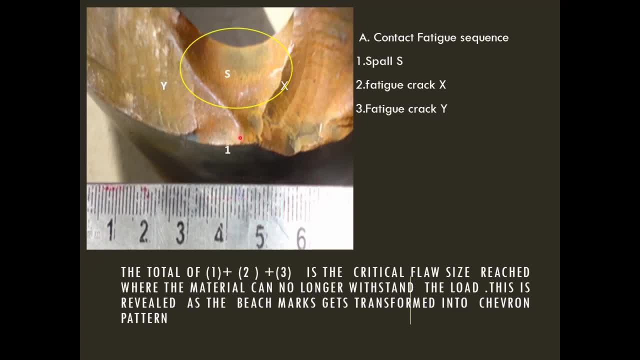 this is the spalled area, and two fields fatigue cracks have propagated simultaneously from the origin of the spalled area here one and this one is two. so this is a somewhat a rapid failure. this fatigue crack propagation in this particular type of failure is very, very rapid, very fast. now let us discuss about something about chivron. 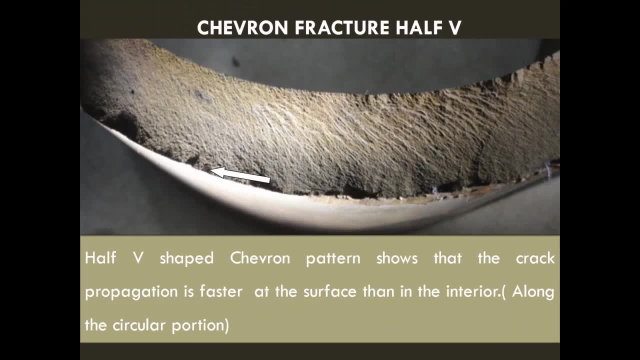 fracture. here you can see half v-shaped fracture. it's not a full v, it's a half v-shaped fracture occurring in a cylinder. see, you can see the lines, or array of lines, traveling from one particular direction only. so this type of fracture is very, very faster than the conventional. 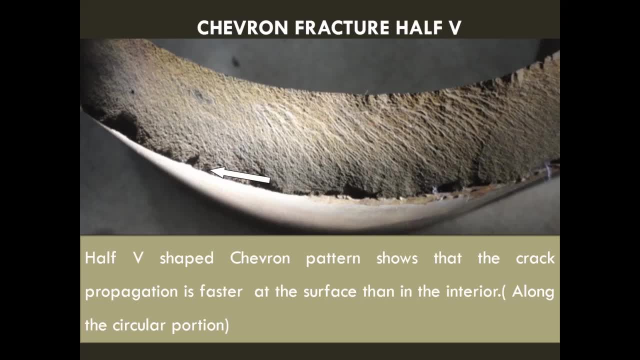 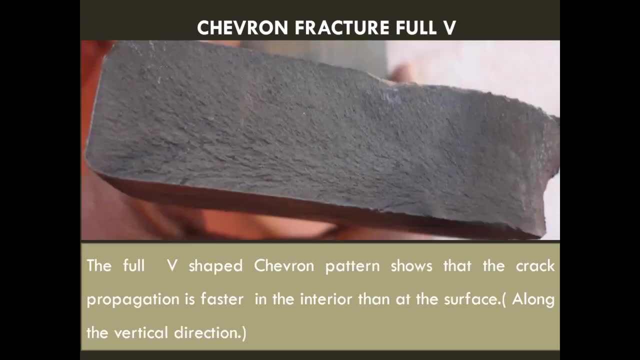 type of chivron fracture that is full v chivron fracture. so this is a fast, rapid fracture. this is chivron fracture full v. the origin of the fracture is here. here the corner is very, very sharp. hence the design problem is there in this particular material. 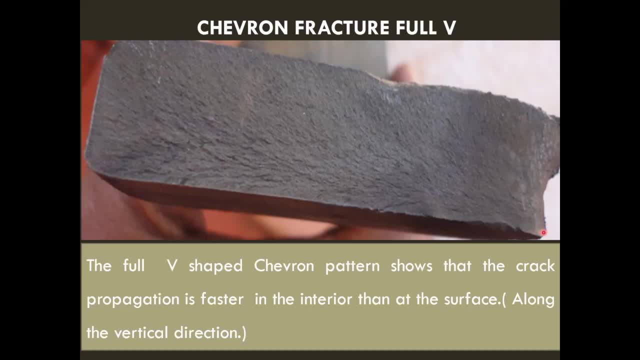 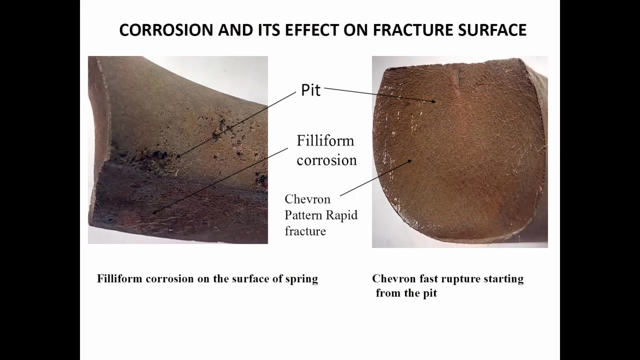 so, since the it is a corner, is very, very sharp. the chivron fracture starts from this particular portion and then radiates in the form of v-shaped fracture, and this is the bottom of the chivron fracture. there are some fractures which are highly influenced by corrosion. see here. normally you 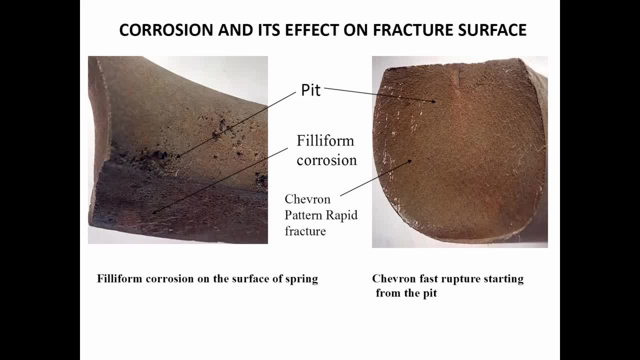 can see in, springs will fail because of fatigue fracture. only here this is a different case. a spring has failed because of a brittle fracture, a chivron fracture. how come see here lot of pits are there on the surface of the spring And they are called as filliform corrosion. 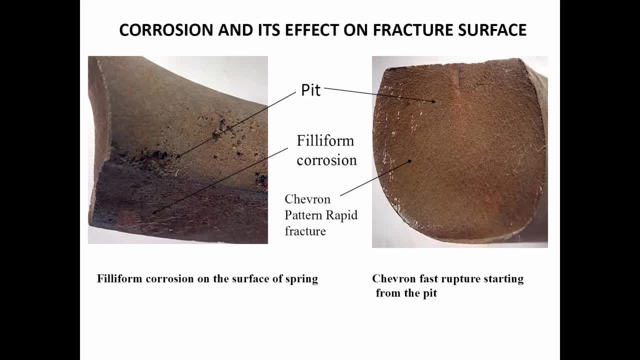 This type of corrosion is called filliform corrosion And you can see there is a pit here, very a pit of very larger size. So this is a pit of very larger size And from there you can see a Chivran, fast fracture emanating from the pit. 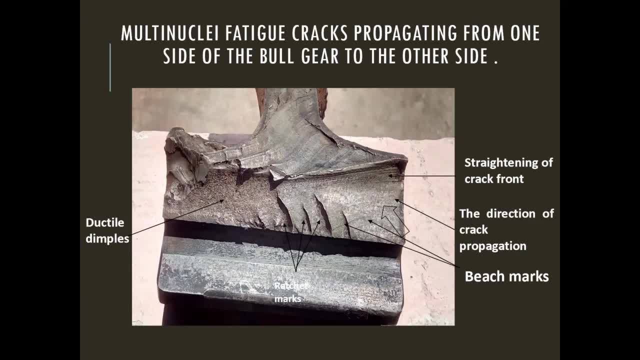 This is a case of multi-nucleic fatigue crack propagation In the. in a case of a bull gear, the crack is propagating at a very faster rate. It starts from the trough of the gear and it's progressing towards the center of the. 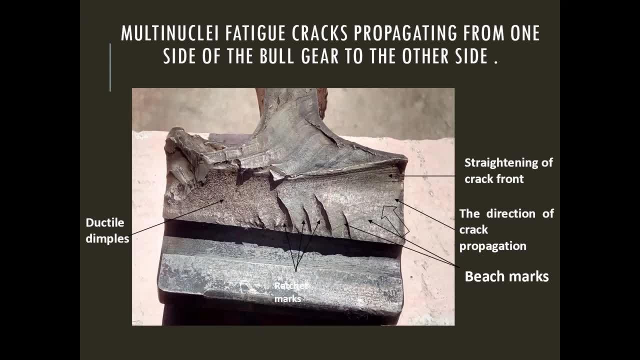 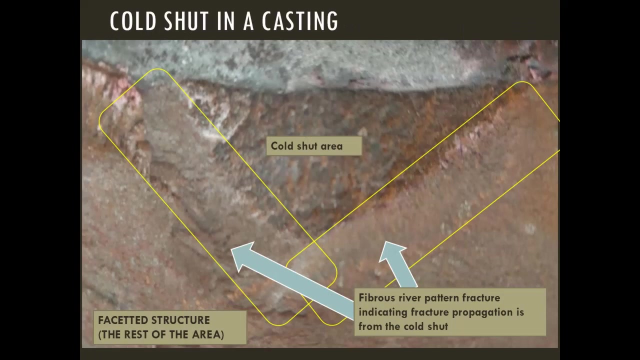 gear in such a way that you can see lot of ratchet marks. See, lot of ratchet marks are seen: One, two, three, four, five, so lot of ratchet marks are there. These ratchet marks are individual fatigue converging at a particular point. 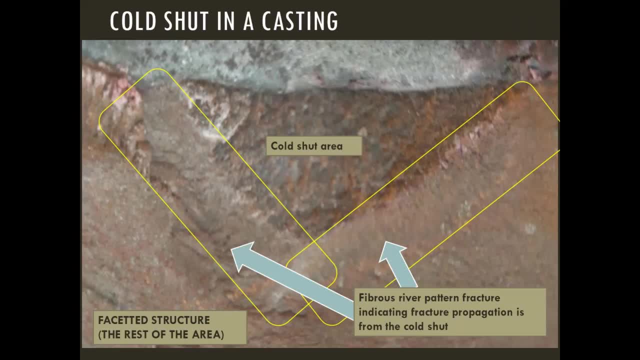 Cold set in a casting is revealed by the fracture feature of river pattern. See here you can see a river pattern emanating from the cold set area. So this is the cold set area, Oxidized area And from the oxidized area you can see fibrous river pattern emerging from the cold set area. 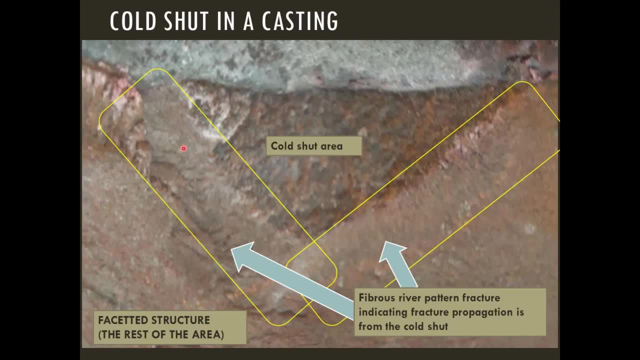 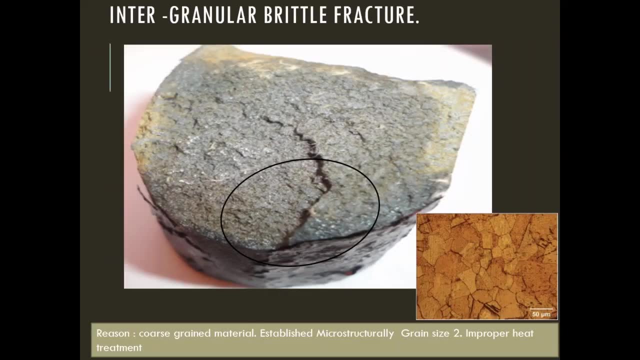 So from this you can conclude that this failure is due to the manufacturing defect called cold set Intergranular brittle fracture. Here the surface is highly crystalline. A zigzag crack starts propagating from the surface. It penetrates deeply into the material. 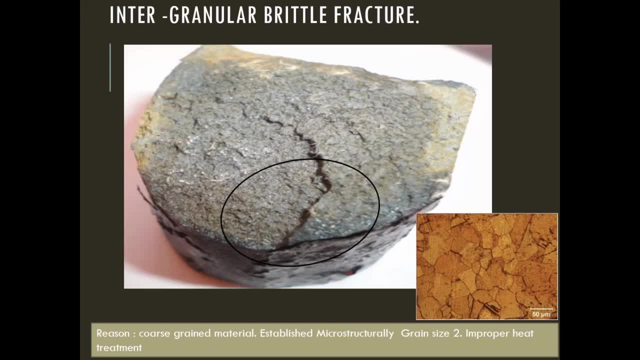 When a piece of sample is cut and examined in a microscope, the grain size was found to be ASTM. grain size two- Normally steel samples having very large grains of ASTM one, two or three, they won't support any load. It will eventually break. 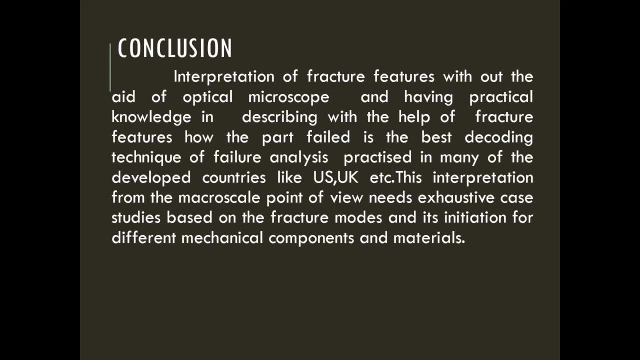 So conclusions, conclusions: interpretation of fracture features without the aid of optical microscope and having practical knowledge in describing, with the help of fracture features, how the part failed is the best decoding technique of failure analysis practiced in many of the developed countries like us, uk, etc. this interpretation from the macro scale point of view needs exhaustive case studies.